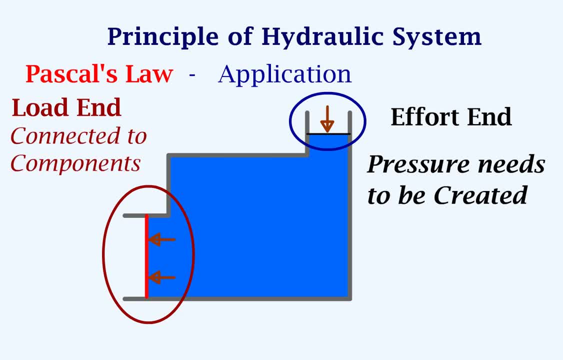 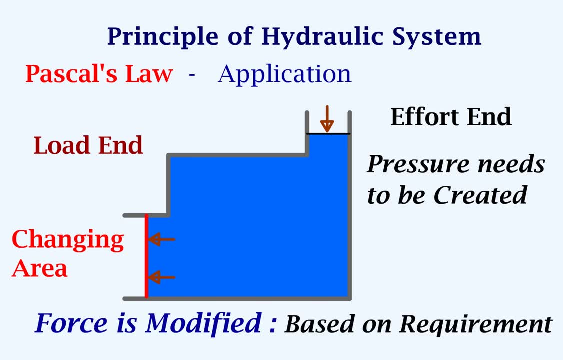 load end, which can be connected to different components that need to be moved. By changing the area at the load end, the force is modified depending on the requirement. With this principle, now let's look at the airplane's hydraulic system by going through the components that form the 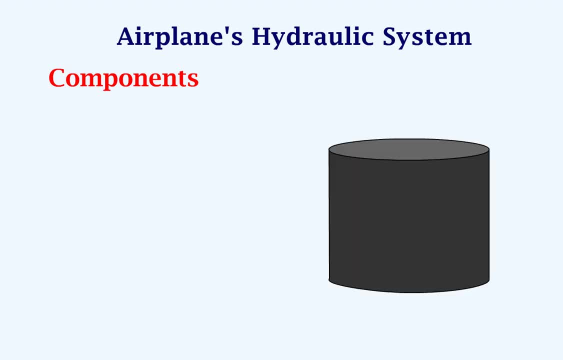 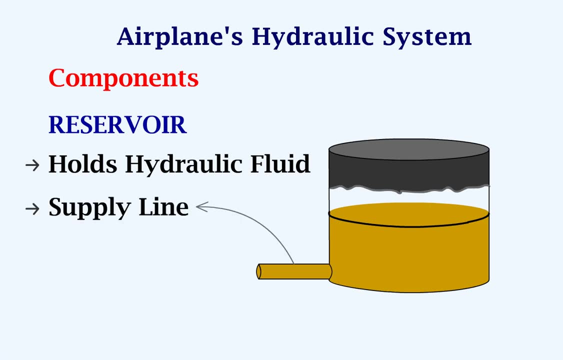 system. Every hydraulic system should have a reservoir. The reservoir holds the hydraulic fluid which is needed for the system. This is the supply line which supplies the required fluid. This is the return line in which the fluid comes back to the reservoir. The reservoir. 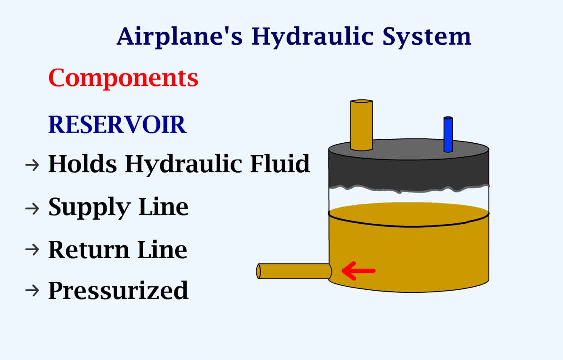 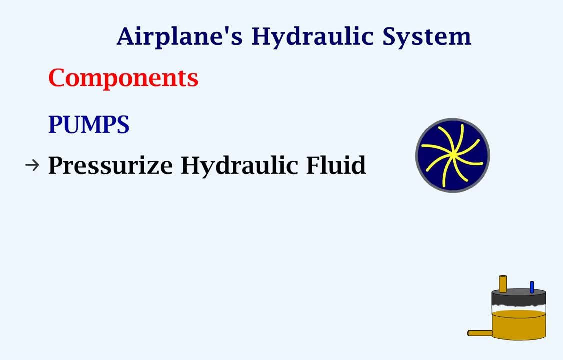 may be pressurized so that a positive flow is maintained on the supply line. The pressurization can be done by taking bleed air from the engine or the APU. The next component we will look at is the pumps. Pumps are used to pressurize the hydraulic fluid. The pump could be driven by. 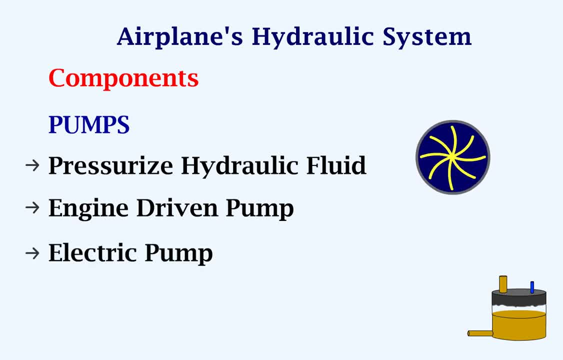 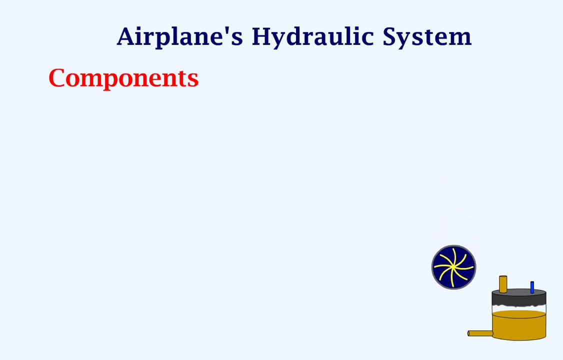 the engine or could be an electrically operated pump. A hand pump may be provided in case engines and the electrical supply is not available. During normal operation of the pump, it must be able to deliver fluid at constant pressure. The next component we will look at is the filters. Filters are used to remove any particles or impurities from the 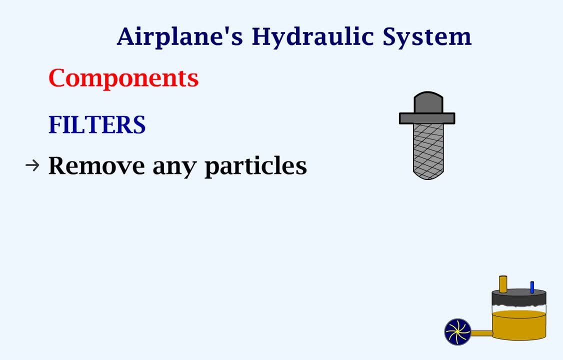 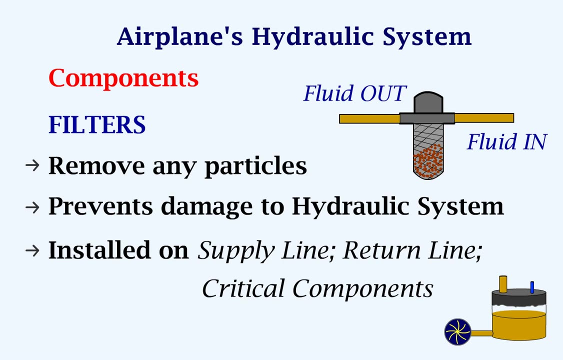 fluid. This is important because it prevents damage to the hydraulic system. They can be installed on the supply line, the return line and also before critical components. As the fluid enters and leaves the filter, the impurities in the fluid get collected in the filter. The next component we will look at is the valves. Valves are used to: 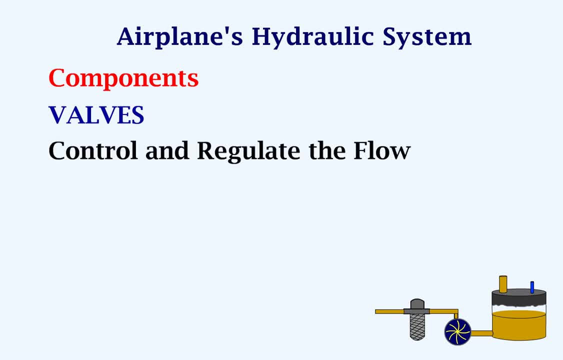 control and regulate the flow of the fluid. There are different types of valves that are used for different functions. First we will look at check valve. The check valve allows the fluid to flow in one direction. only If the fluid enters from this side it is allowed. 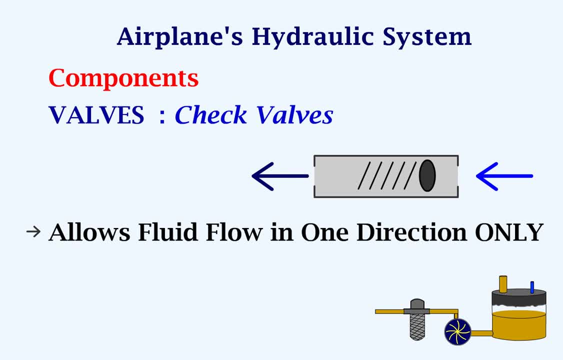 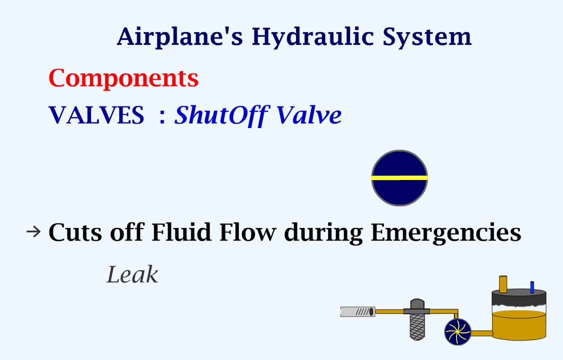 to flow to the other side. If the fluid enters from this side, it is allowed to flow to the other side. Next we will look at shut off valve. This valve cuts off the hydraulic fluid from the system during emergencies such as leak, fire or a pump fault. When this valve closes, it prevents the fluid.